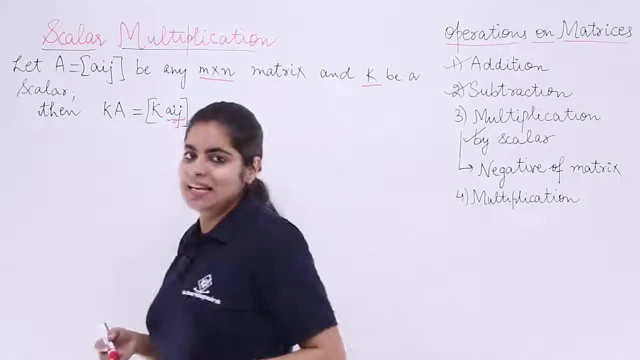 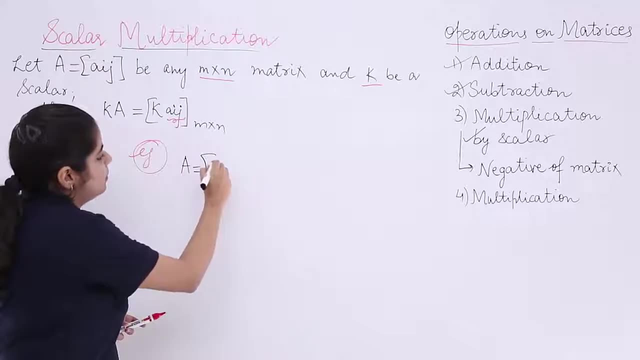 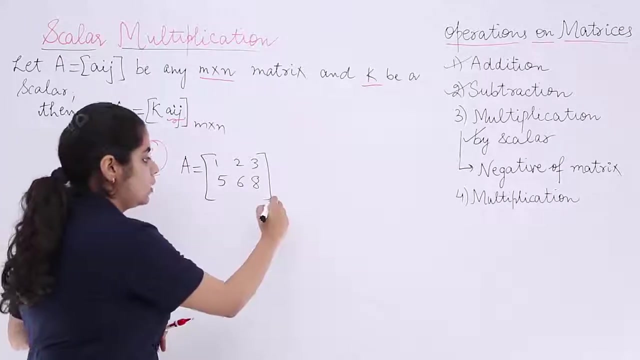 That's it Still not understood. Let's see the example. The example for that. I take a matrix, say, given to me is a matrix a, and that matrix is something like this: What is the order? There are how many rows? There are 2 rows and 3 columns, So it is a 2 by 3 matrix. 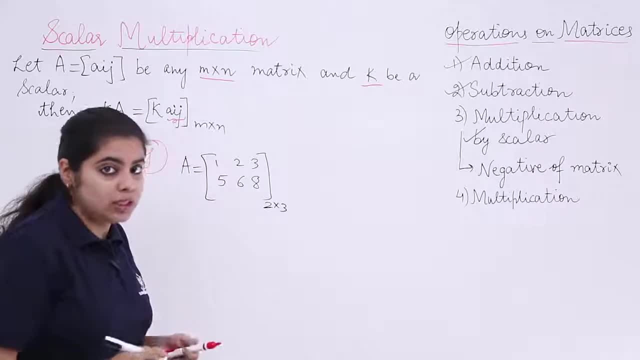 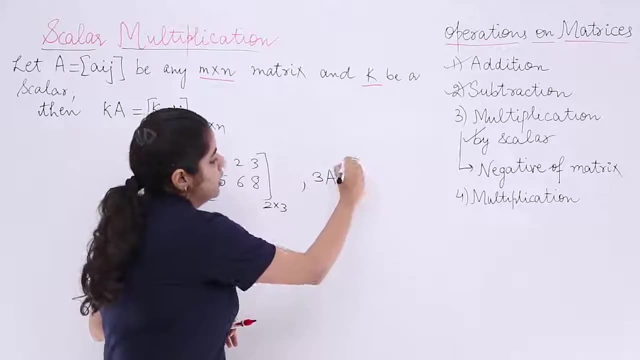 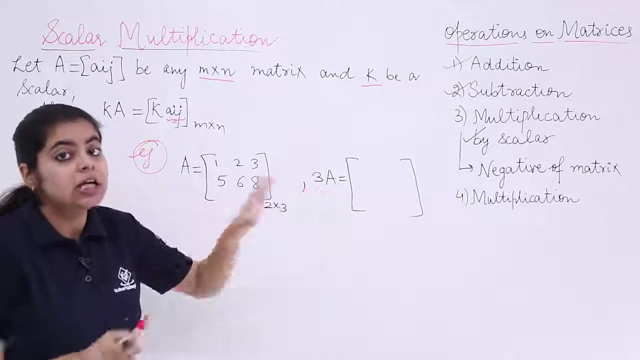 Now, if given to me is a scalar 3 and I have to compute 3 of a, Now I am supposed to find out 3 of a. One thing one should keep it in mind: multiplying by a scalar does not change the order. Remember, there was m by n earlier. there is m by n here also. That means the order remains same. 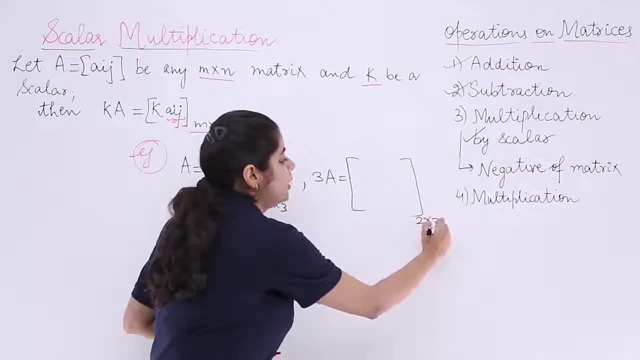 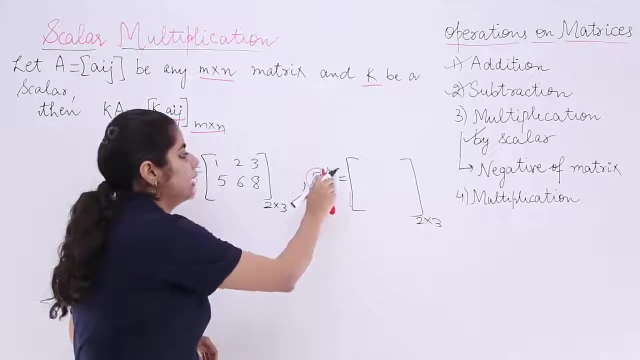 So if it is 2 by 3 here, it will remain 2 by 3 here, only. That means 2 rows, 3 columns. Now what is the scalar? 3 is the scalar? That means you have to multiply the whole matrix a. 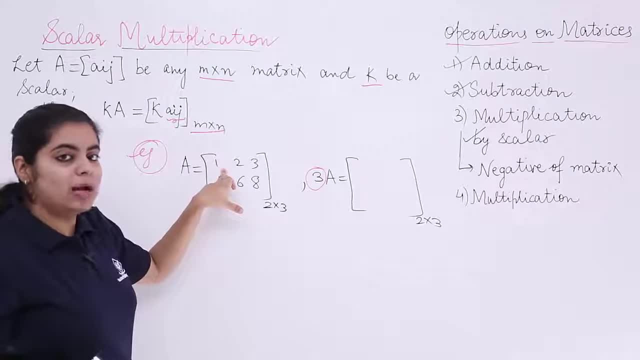 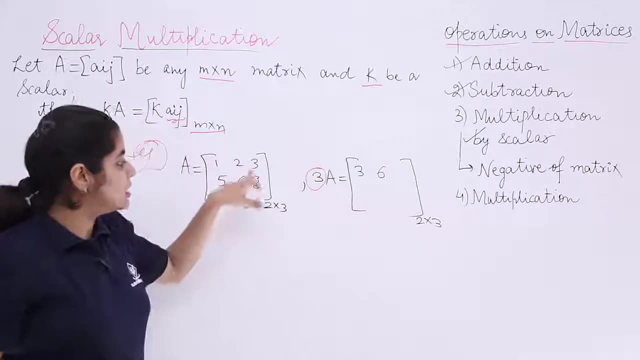 By that constant scalar 3.. So multiplying 3 by 1 is giving me 3.. Multiplying 3 by 2 is giving me 6.. 3, 3s are is what 3, 3s are is 9.. First row is completed. 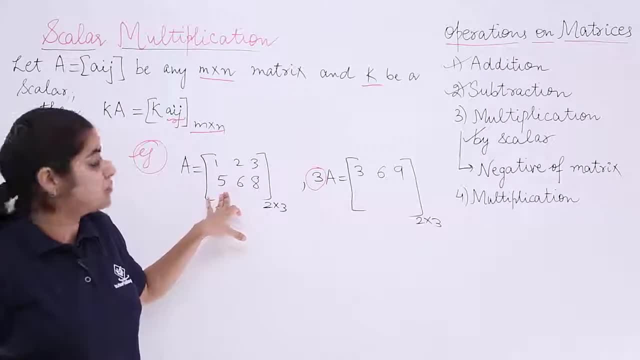 Similarly, now you can go about completing the second row: 3- 5s are 15, 3- 6s are 18.. So it is 15 and 18 and last but not the least element is what? 3 8s are 24.. So that means what That means. if I need to multiply by a, I have to multiply by a. 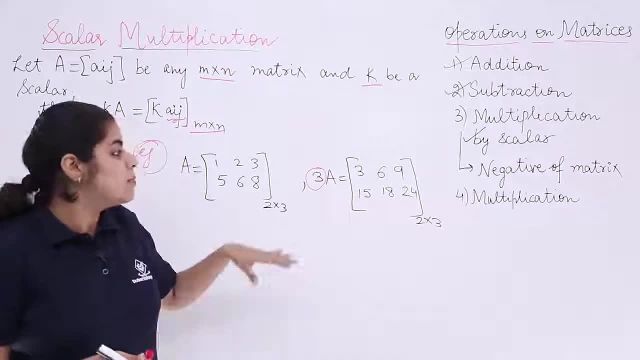 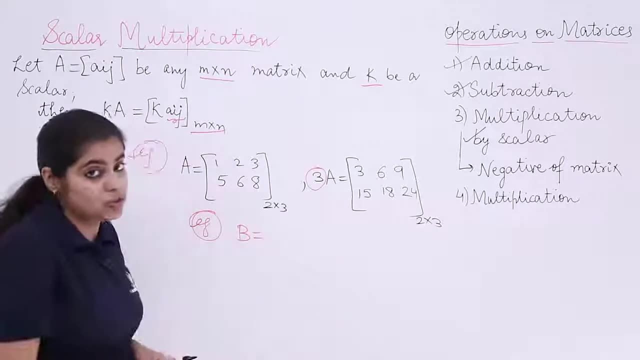 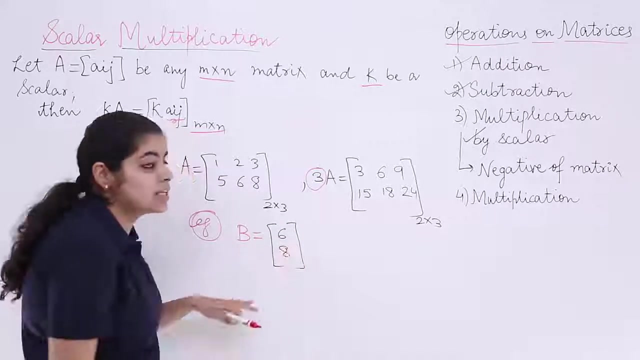 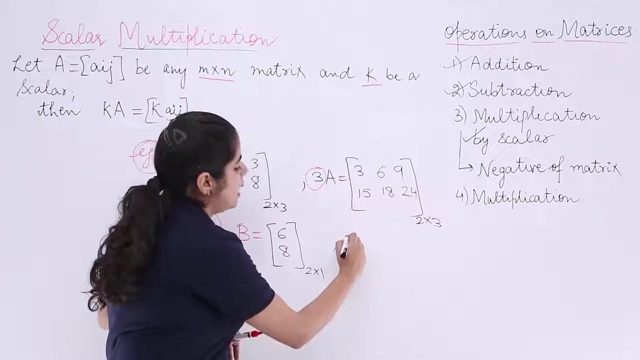 By a scalar quantity. I don't need to disturb myself much because the order is same. Suppose we take another example for your convenience. Example: is a matrix given to me which is b. The matrix is a column matrix, So it has how many rows? It is given to me that it has 2 rows, So it is 2 rows and 1 column. Now I am supposed to find out what I am supposed to find out. say 2 by 4 of b.